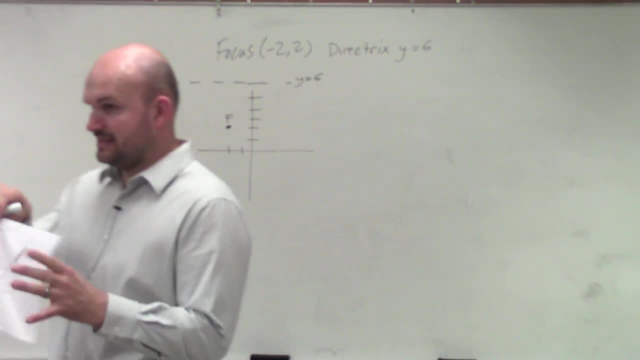 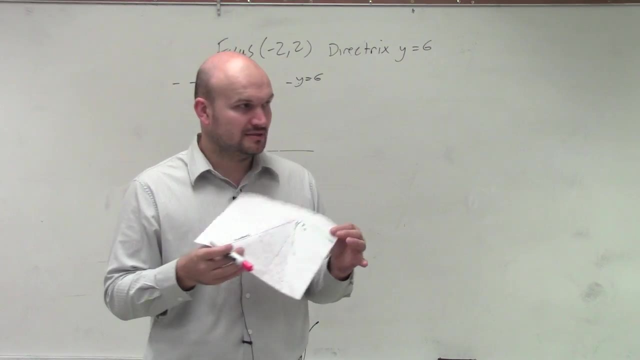 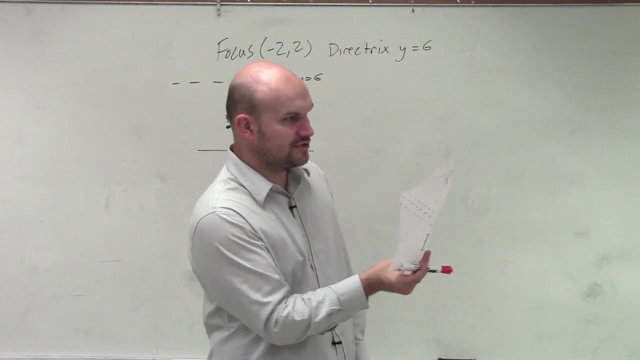 if you kind of forget, which a lot of students do, think back to this or keep this: If you're given your focus and your directrix right, your parabola goes towards your focus and away from your directrix, right. Somebody say that Goes away from the directrix the line that purple. 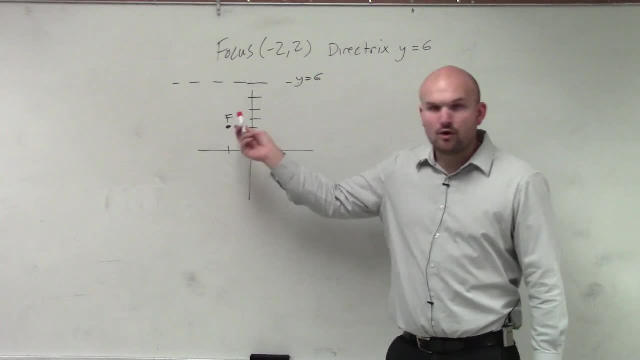 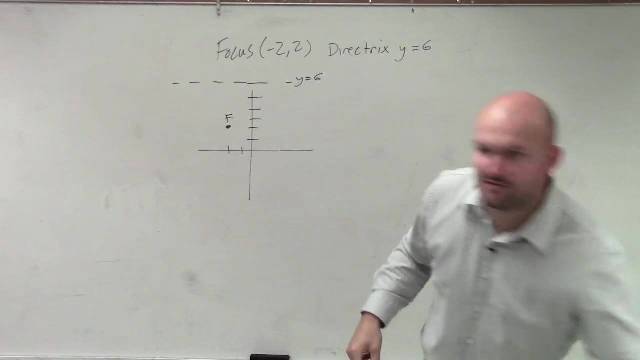 line and it goes towards your focus. So is this going to be a horizontal or a vertical? Is it going left and right? No, it's going down right. I don't know what the graph looks like, but it's going to be a horizontal or a vertical. So if you're given a focus and your directrix- 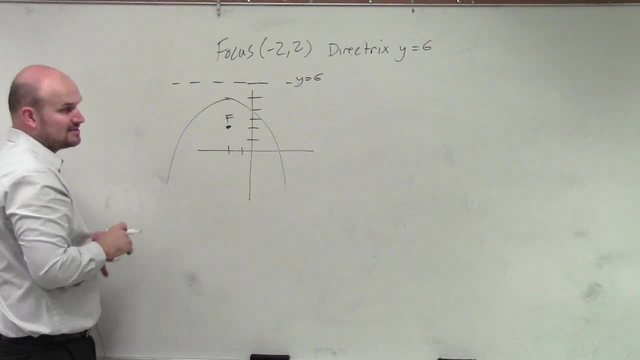 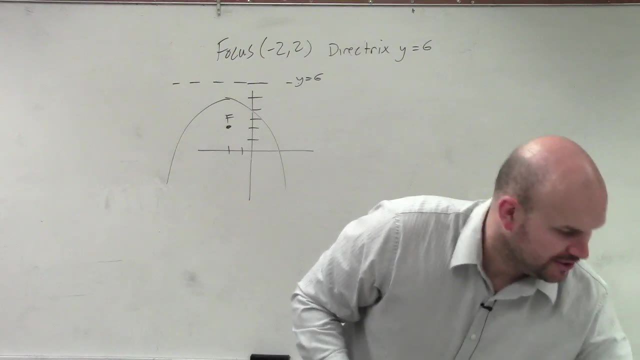 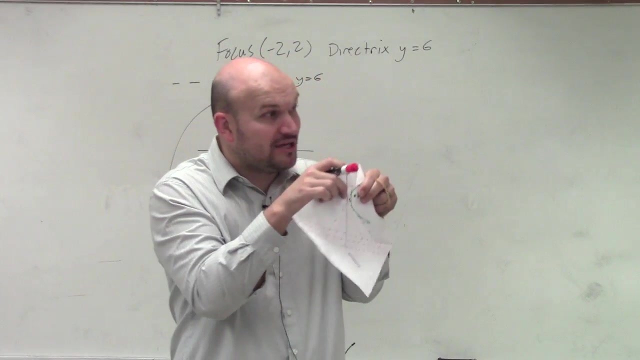 it's going somewhere like this, It's going towards the focus. So there's a couple things we also need to remember. Also, in addition to that, your vertex, which we need to figure out because we need to know what h and k is. your vertex is in between. It's in it's right, in the 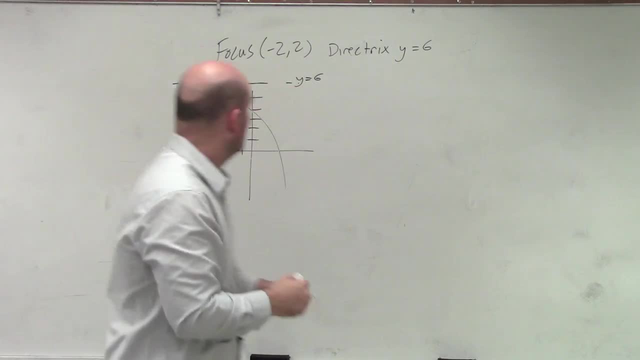 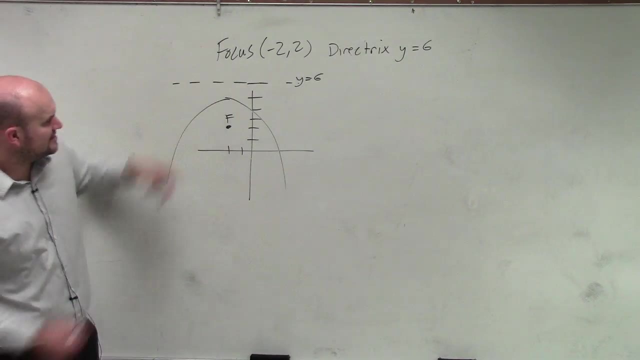 middle, Right in the middle. So can we find the, can we find the middle distance between our focus and our directrix? Yeah, just let's see. One, two, three, four. Oh, it's right at two. 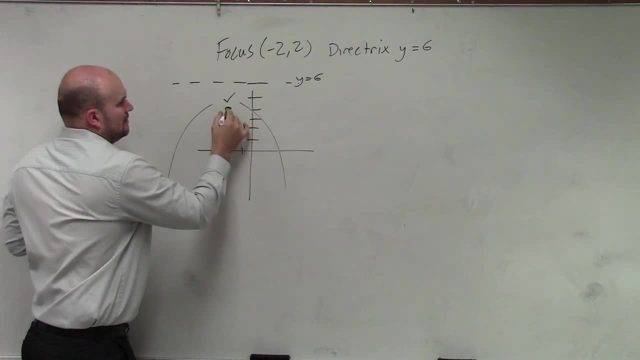 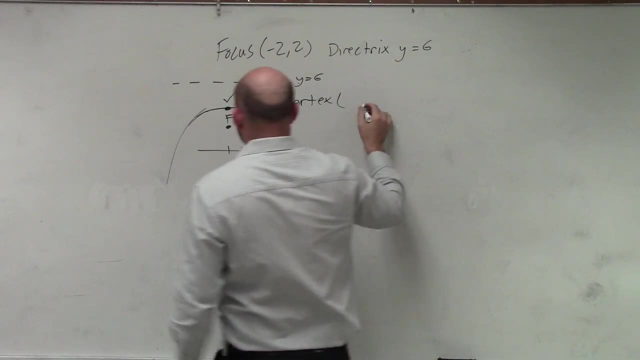 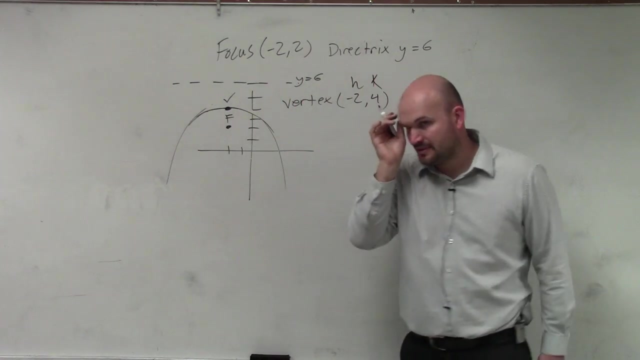 That's my vertex. It's actually right there. So what is that point? So my vertex is at negative two, one, two, three, four. That's important because that's my h and that's my k. Now, if my 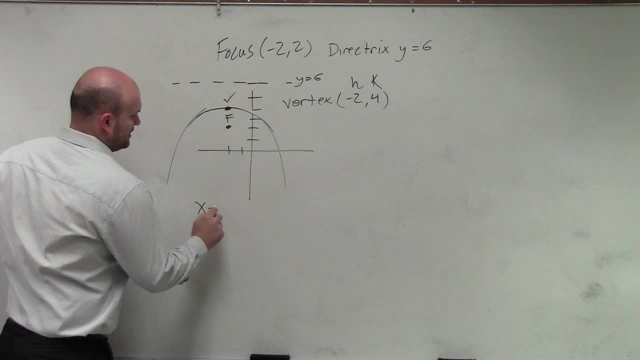 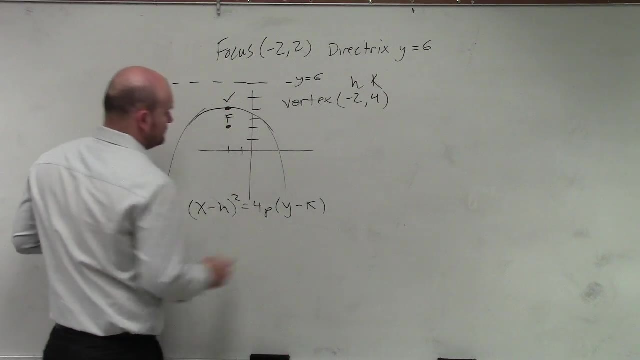 horizontal looks like this. here's what my vertical looks like. It's just the exact opposite, but my h is squared. And then again, remember, Daniel, that h always goes with x, y always goes with k. I will mix it. 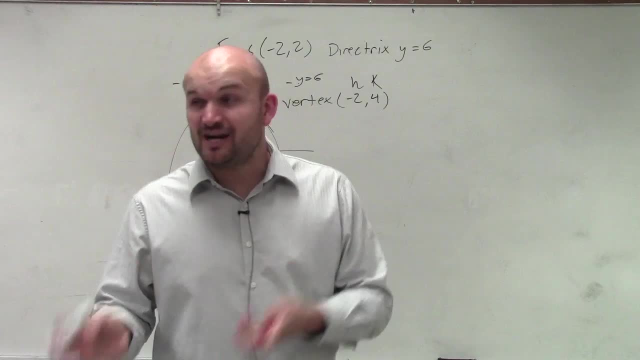 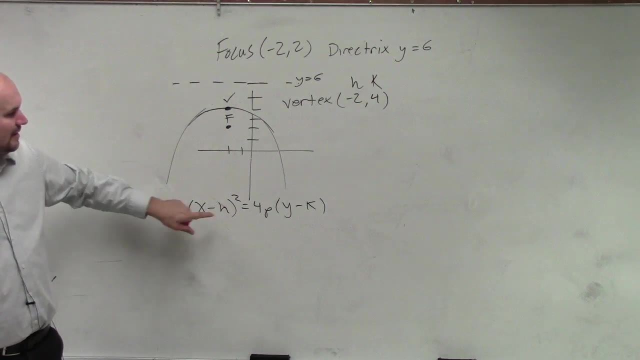 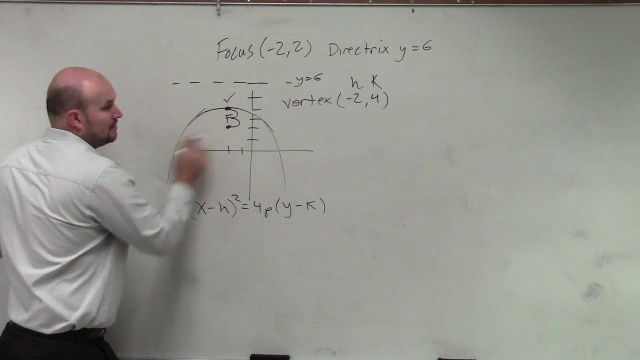 up. I have some videos where I make that mistake, Nick. So we've got to be careful that we don't do like the other mistake. So you basically need to know those two equations And then we need to figure out p. So p is the distance from our vertex to our focus, which is how far Two? but 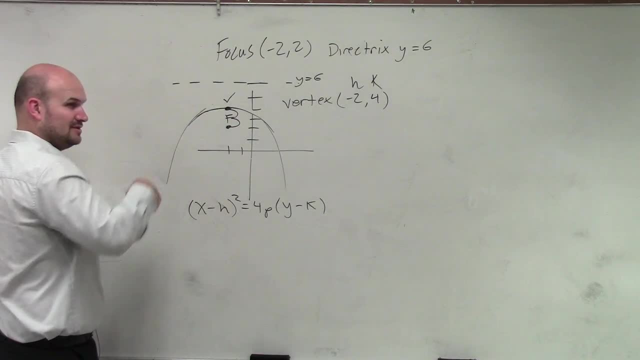 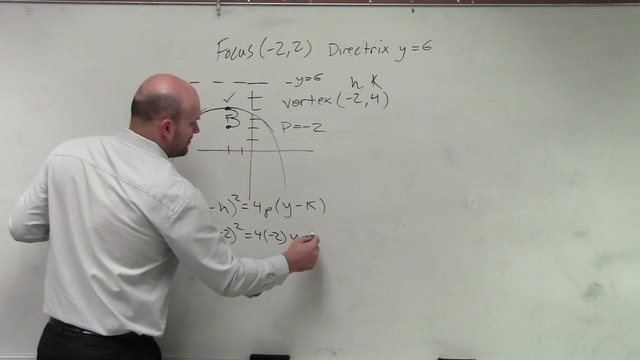 it's going down. So therefore it's in the positive or negative direction. So it's going in the negative direction. So you would say p is equal to negative two. So x minus a negative two squared equals four times negative two. y minus four. Does everybody see how I plugged?